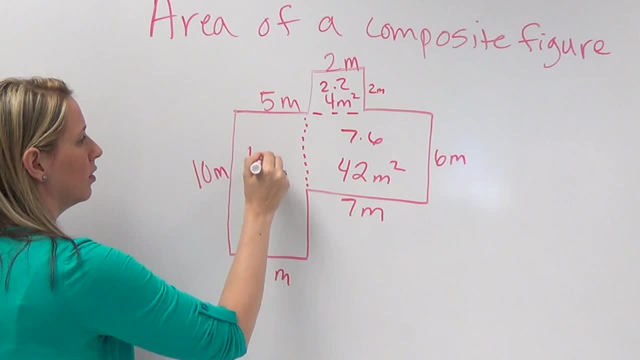 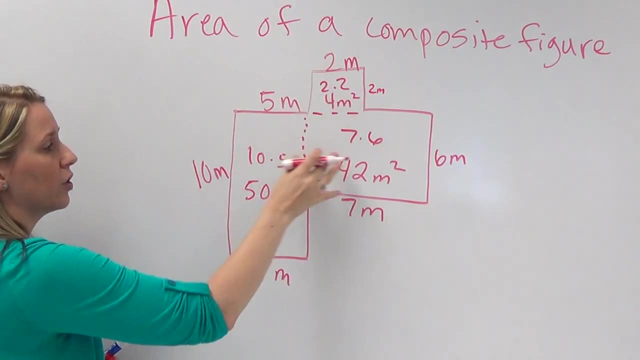 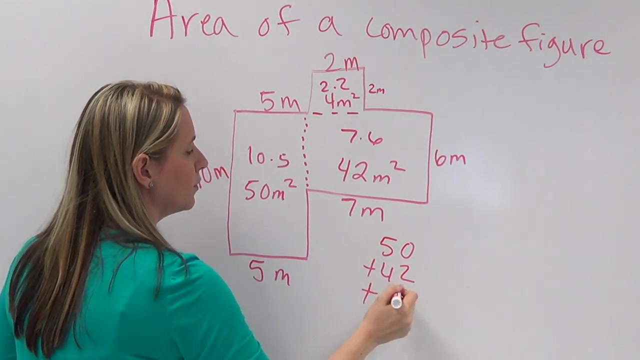 another rectangle here Ten times five is going to give you fifty meters squared. Now we've got each of our little sections, So to find the area of the whole thing you just add them all together. For example, fifty plus forty-two plus four is going to give 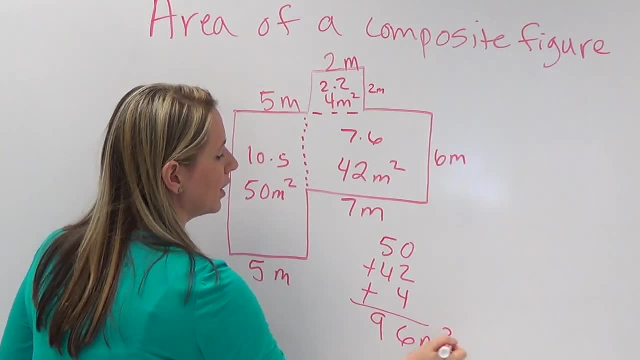 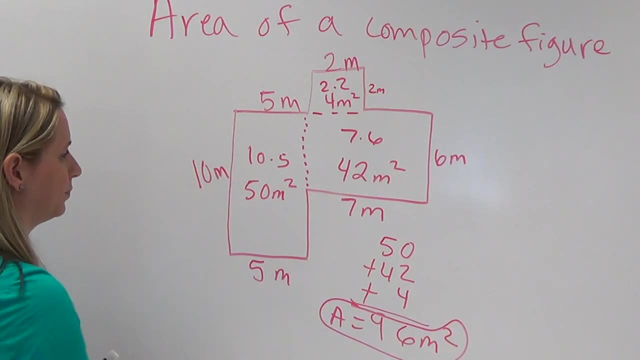 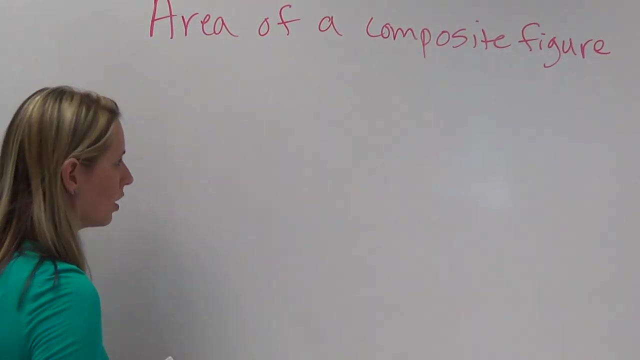 you ninety-six meters squared, Subtitles by the Amaraorg community, and that would be the area of the whole figure. Let me show you another one. Let's say we had something that wasn't quite as simple to see. Let's say you had something like this: 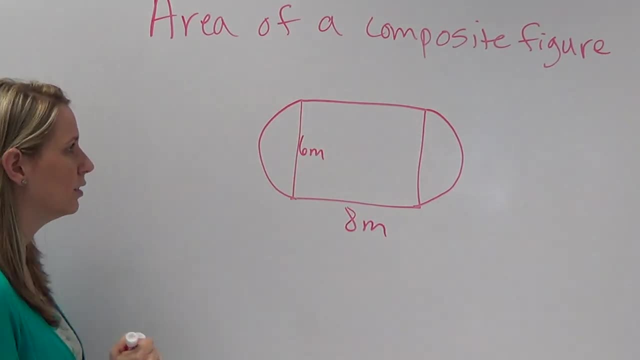 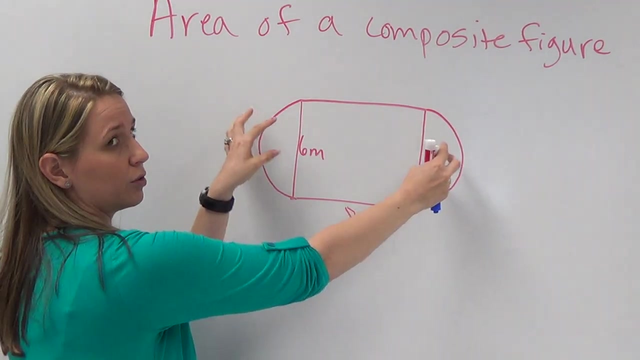 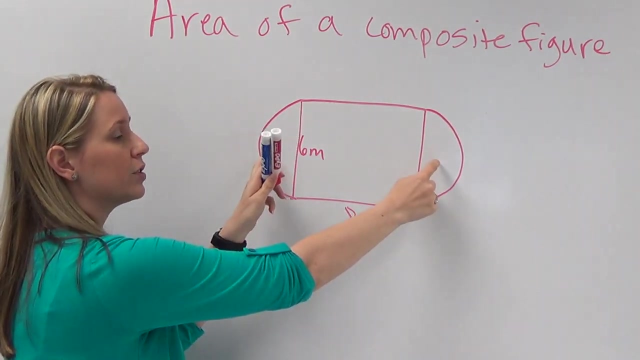 Okay, here we have two semicircles and a rectangle, So what we really need to do is take the area. If you put these two semicircles together, you get one circle and then you've got a rectangle in the middle. So we need to take the area of the rectangle and the area of the circle. 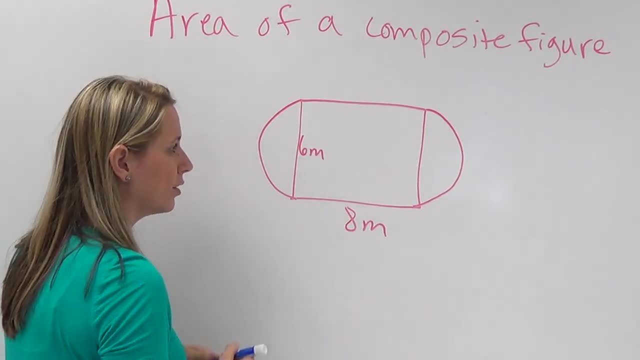 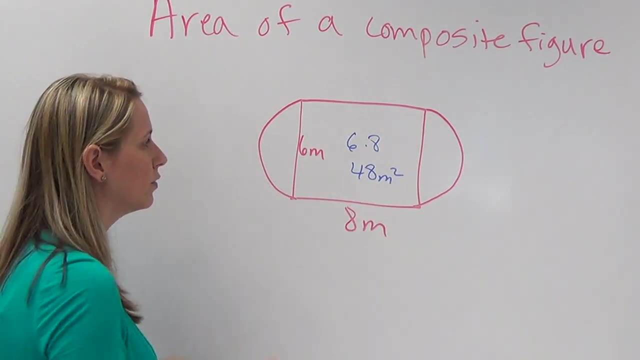 which would be the two semicircles put together. So the area of the rectangle would be six times eight, which would be forty-eight meters squared. Now you may wonder, for this circle or semicircle, the area of the circle is pi times the radius squared. Well, I don't. 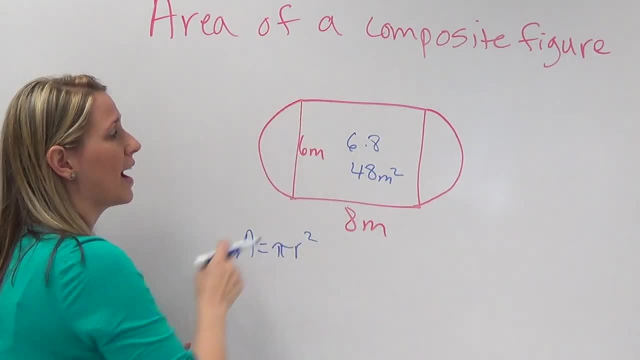 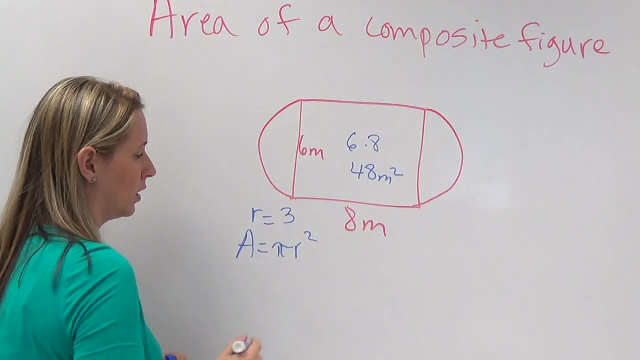 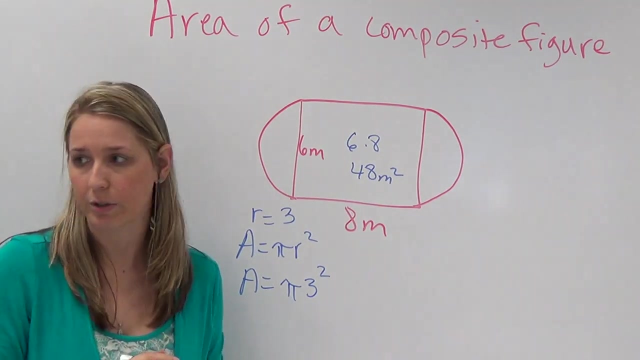 have the radius, but this side of the rectangle is actually the diameter of the circle. So if you divide that by two, it gives you my radius. So my radius is three. So then I just plug that in, So we have pi times three squared, and you can just plug it out in the calculator. 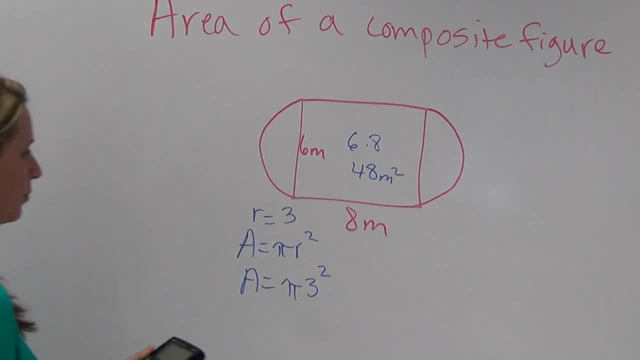 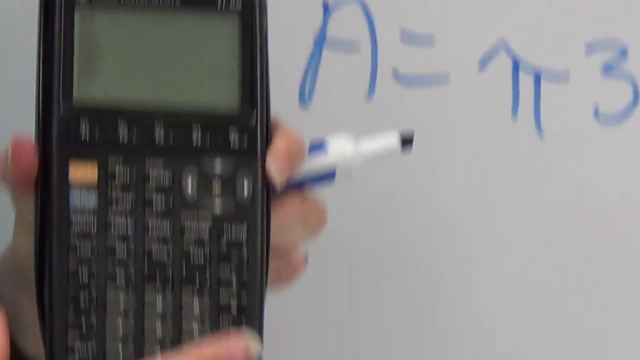 Let me grab it. Subtitles by the Amaraorg community. So we have pi is right above the housetop, So we get second housetop. That gives us pi times the radius, which is three squared. So we have pi, three squared. Hit enter And. 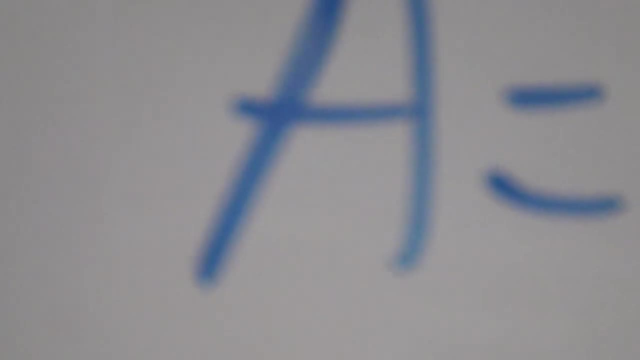 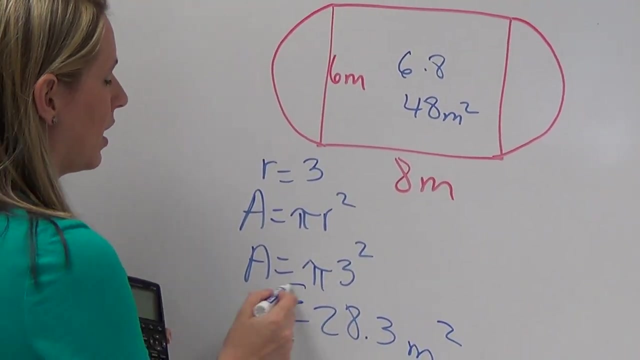 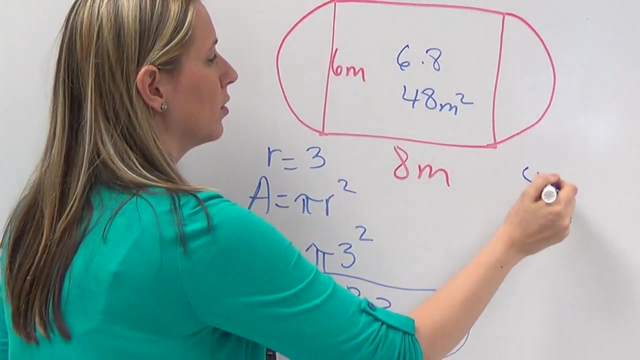 that's going to be about twenty-eight point three. So twenty-eight point three meters squared. So now we have our half circles put together to make a whole circle And we have our rectangles. We just add them together. So forty-eight point three meters squared. 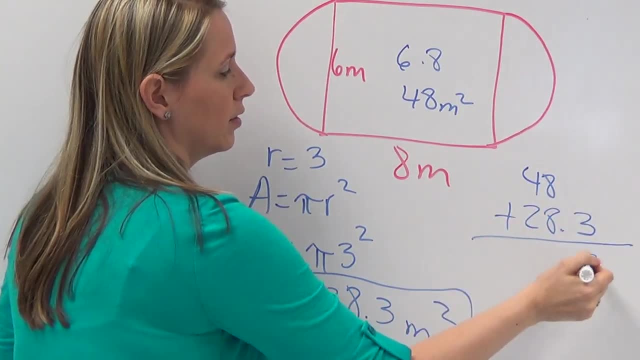 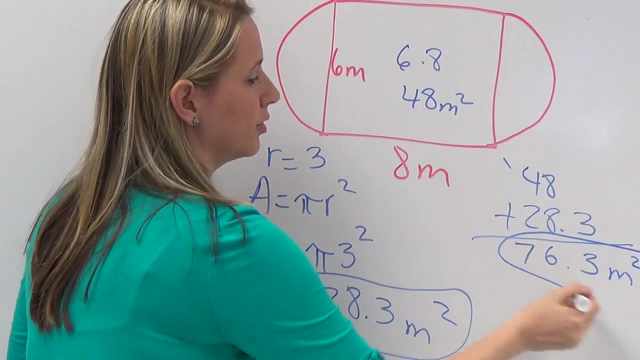 Forty-eight plus twenty-eight, point three is going to give you about seventy-six point three meters squared, And that's how we do. area of a composite figure.